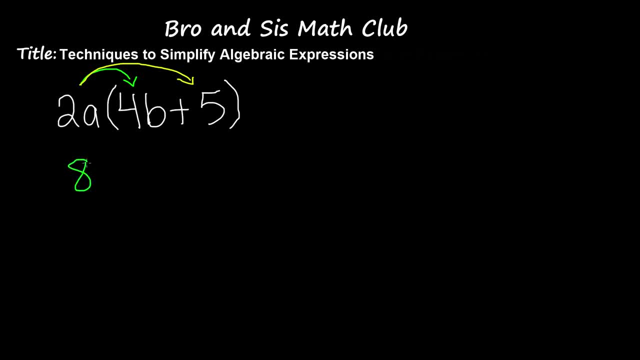 2a times 4b gives us 8.. 8a b. 2a times 5 gives us positive 10a. This is the simplified form of this expression. Now let's simplify this algebraic expression. So remember to simplify an algebraic expression. first you have to apply the distributive property where it needs to be applied. 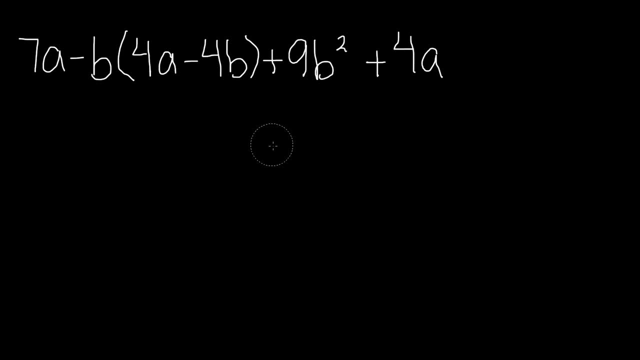 and then you find the like terms: Add or subtract them. This part of the expression is where we can apply distributive property Negative b, parentheses 4a minus 4b. First let me just copy this term down: 7a. 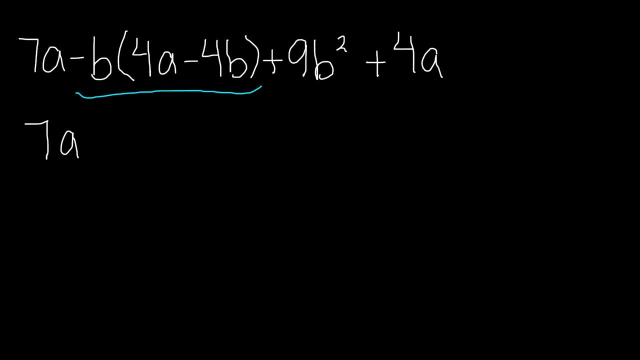 Now we solve- We need to solve this using distributive property. So we're going to multiply first negative b Times 4a, And then we're going to multiply negative b times negative 4b. Negative b times 4a gives us negative 4ab. 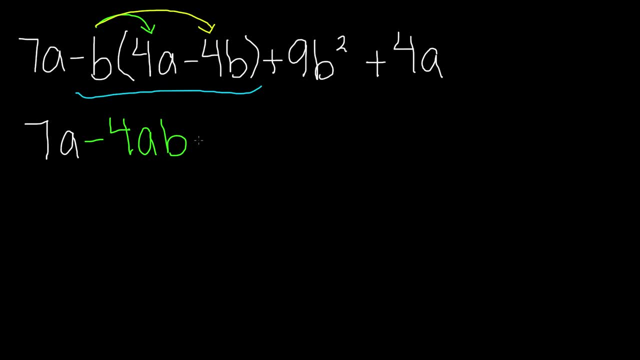 Negative b times negative 4b gives us positive 4b to the second power. Now we copy down the other terms which are positive: Negative: 9b to the second power plus 4a. Second step is to find the like terms and add or subtract them. 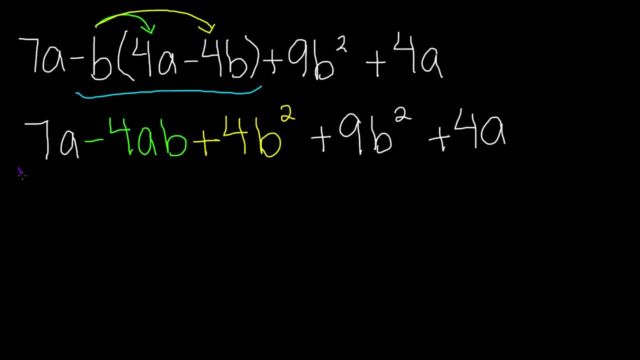 So our first like terms are 7a and 4a. Why are they like terms? Well, because like terms are terms that have the same variable and the same power of that variable. So a doesn't have a power, So the power is going to be 1.. 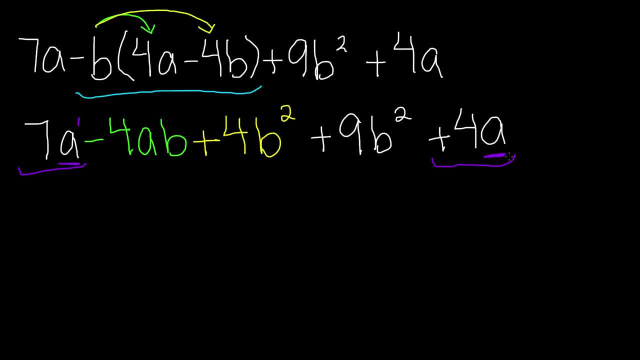 In the same way, 4a, a is the same variable And it has the same power, which is 1.. So 7a and 4a make 11a, And then now you copy down the term which is negative, 4ab.